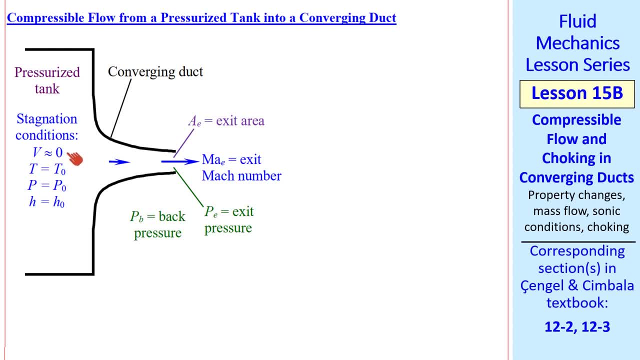 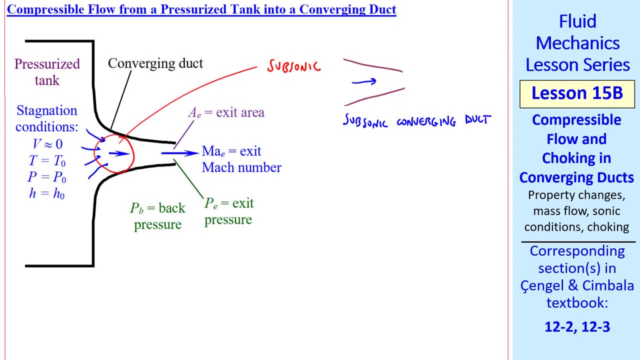 Now let's think about this flow. It starts at zero speed and accelerates into the converging duct. The flow here has to be subsonic And, as discussed in a previous lesson, for a subsonic converging duct, speed goes up, Mach number goes up. 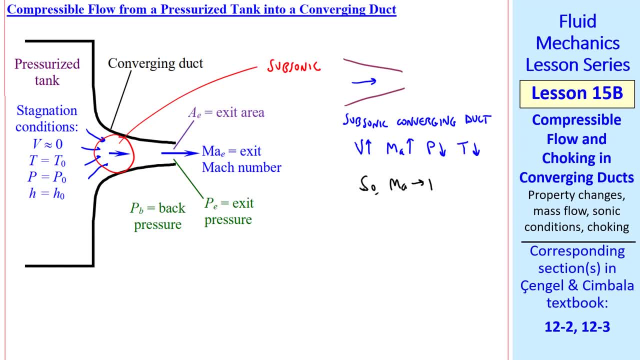 pressure goes down And temperature goes down. So while the flow is subsonic, the Mach number is approaching one. Now suppose that here the Mach number becomes greater than one, In other words supersonic. Well, for a supersonic converging duct the behavior is opposite. 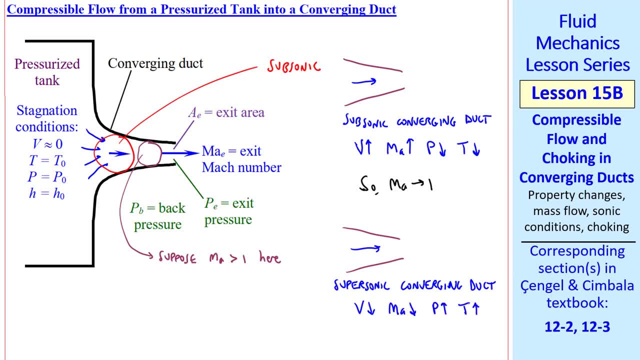 So V and Ma go down, Pressure and temperature go up. So as soon as the Mach number is greater than one, it has to start going back down. Well, this doesn't make any sense. Therefore, we conclude that the flow cannot go supersonic in this duct. 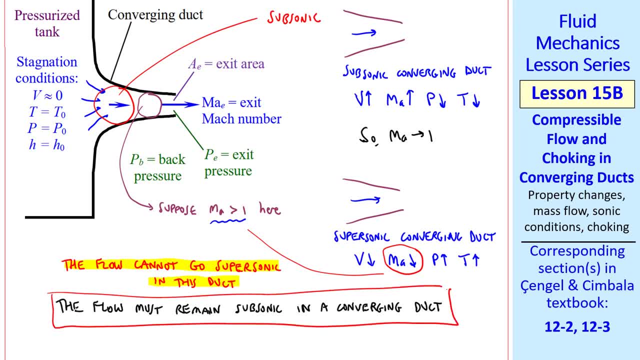 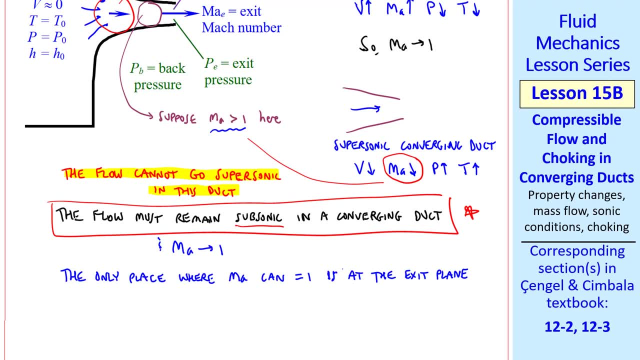 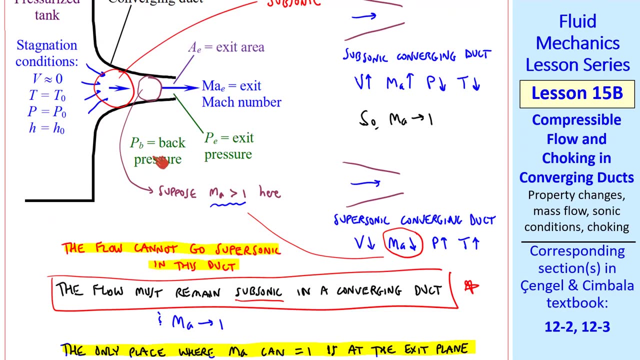 In other words, the flow must remain subsonic in the converging duct, And the Mach number approaches one but cannot exceed one. So we also conclude that the only place where Ma can equal one is at the exit plane. Here's where the back pressure comes in. 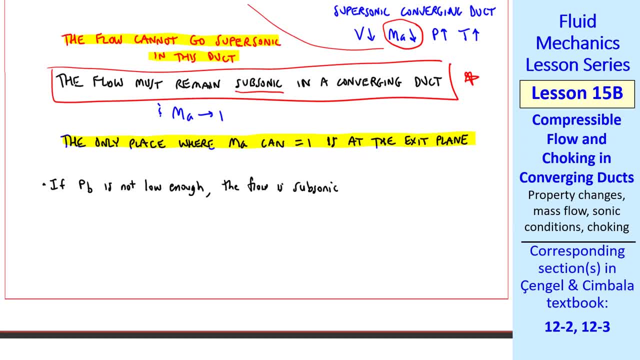 If back pressure, Pb is not low enough, the flow is subsonic and Mach number is less than one at the exit plane. If Pb is low enough, the flow is still subsonic, except Mach number equal one at the exit plane. 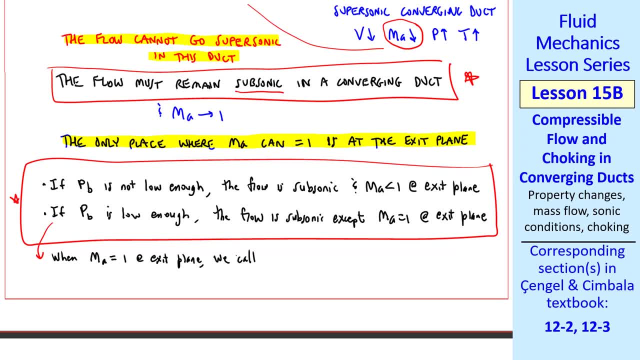 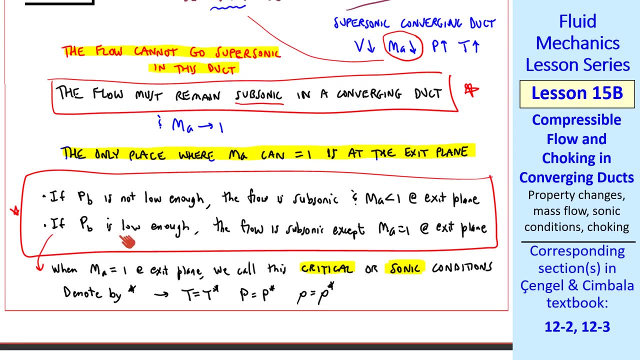 For this second case, when Mach number equal one at the exit plane, we call this critical or sonic conditions And we denote this by an asterisk. So T equal T star, P equal P star, rho equal rho star, etc. But how low of a Pb is low enough? 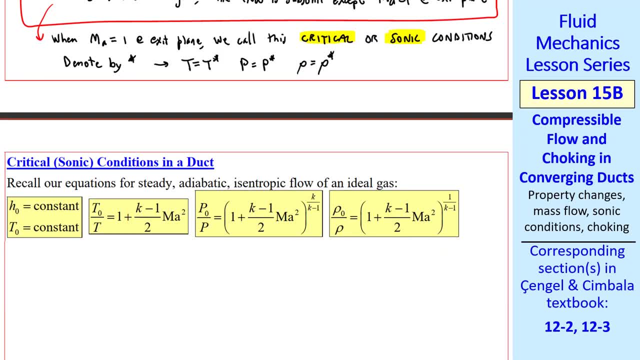 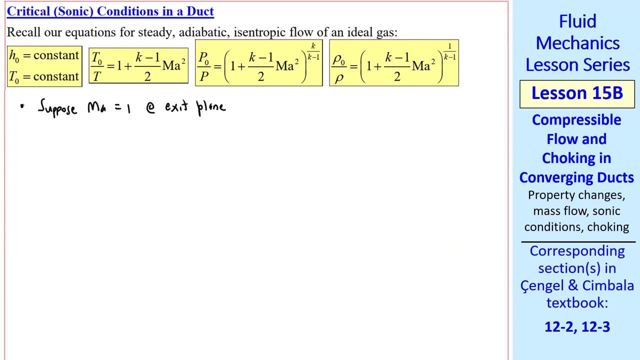 to make the flow sonic at the exit plane. Well, let's go back to our equations for steady adiabatic isentropic flow. Suppose Mach number is one at the exit plane, So let's set Ma equal one in these equations. 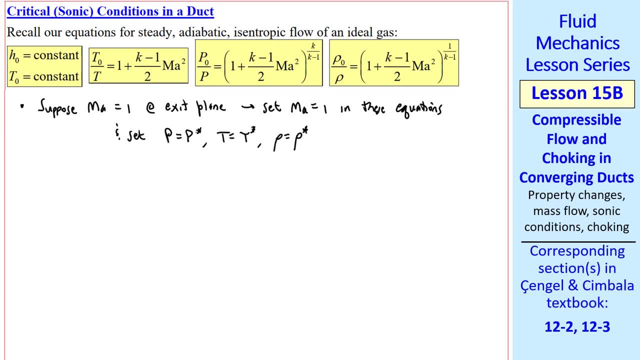 And set P equal P star, T equal T star and rho equal rho star, So these equations become: T naught over T star is one plus K minus one over two times one squared, which is just one, And similarly P naught over P star. 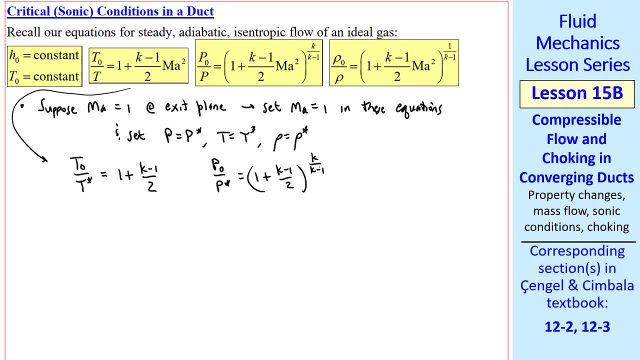 is one plus K minus one over two. To the K over K minus one exponent. And a similar equation for rho naught over rho star. Well, in all the textbooks, people like to calculate the reciprocal of these equations. So we write this as T star over T naught. 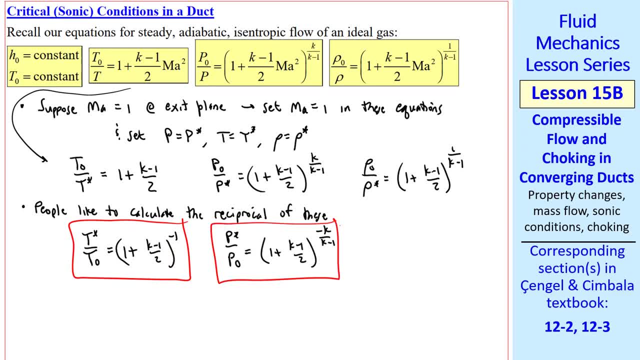 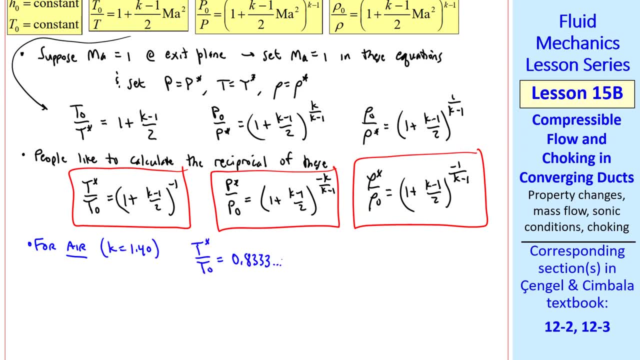 And we simply take this quantity to the negative one. We do the same with pressure and density For air. K is one point four O. So T star over T naught is zero point eight, three, three, three, three, three. One to four digits. P star over P naught is point five, two, eight, three. 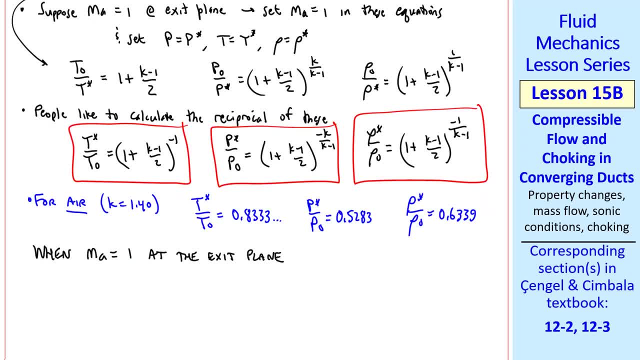 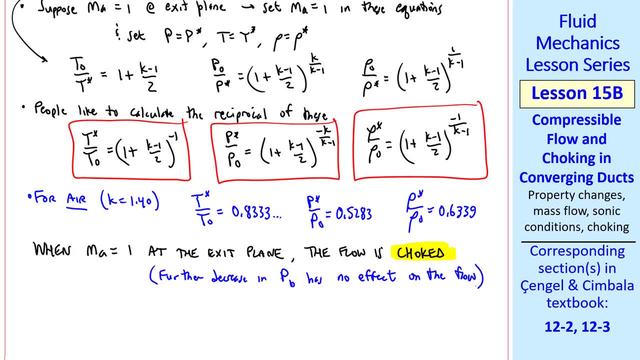 And rho star over. rho naught is point six, three, three, nine. When the Mach number equal one at the exit plane we say that the flow is choked, Which means that further decrease in Pb. the back pressure has no effect on the flow. 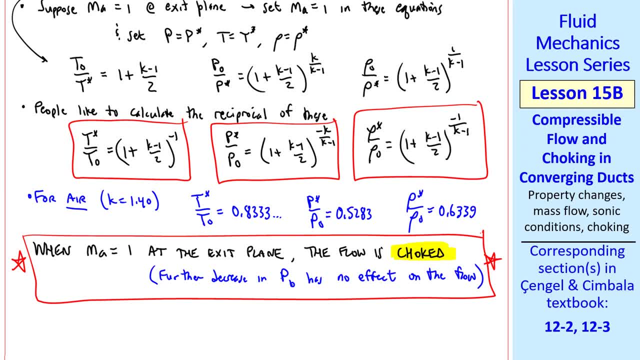 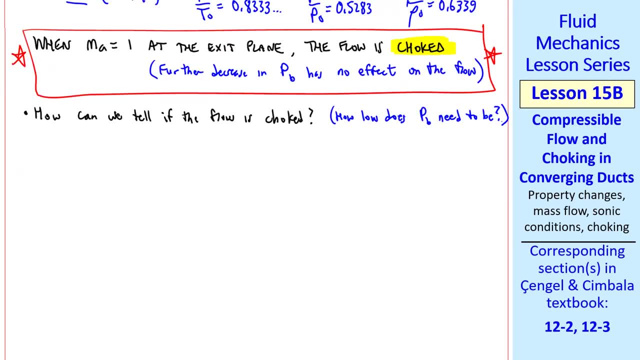 Choked flow is an important concept in compressible flow. So let's go back to our question: How can we tell if the flow is choked? In other words, how low does Pb need to be? I'll give three cases here. If Pb is greater than P star: 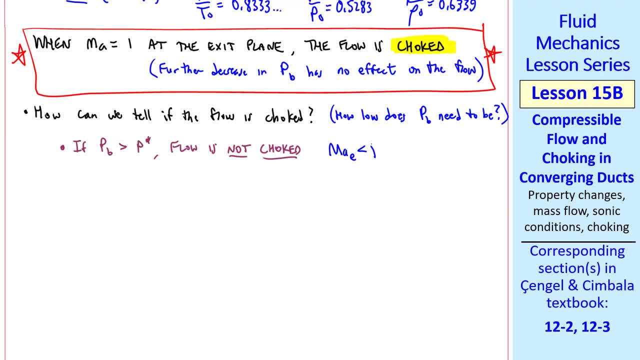 the flow is not choked. Mach number at the exit is less than one And Pe equal Pb, Any subsonic jet exiting into the air has the same pressure as the surrounding back pressure of the air. If Pb equal P star, the flow is choked. 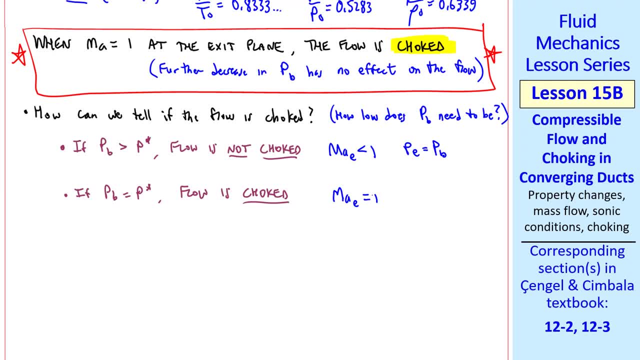 just barely. The Mach number at the exit is equal to one And Pe is still equal to Pb, but is also equal to P star, The critical or sonic condition. If Pb is less than P star, the flow is choked. Ma at the exit is one. 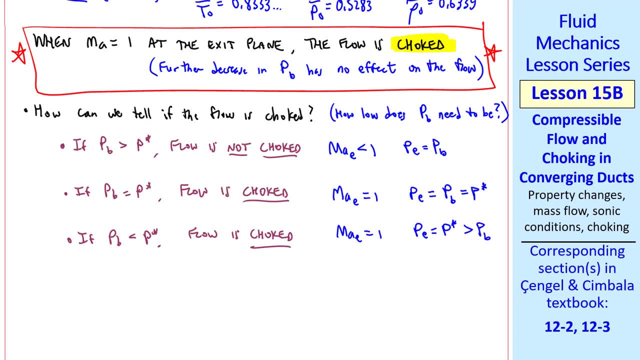 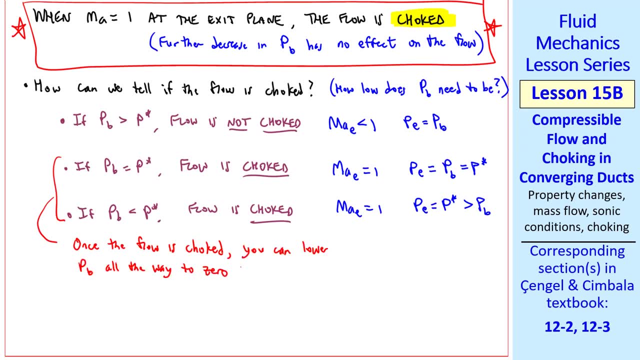 And Pe equal P star, But P star is greater than Pb. as we said here, Once the flow is choked, you can lower Pb all the way to zero. In other words, a perfect vacuum, And nothing in the nozzle will change. 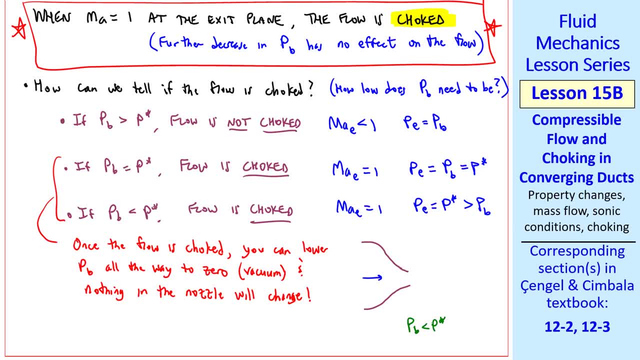 So for any condition in which Pb is less than P star, the Mach number at the exit plane is one. The pressure at the exit plane is P star, Te equal T star And rho E equal rho star, No matter how far you lower the back pressure. 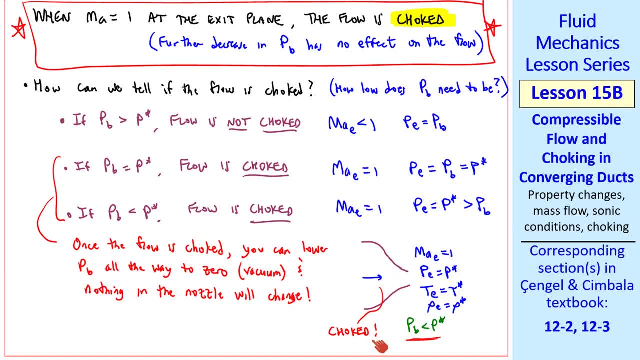 the flow in here remains constant and choked. Why? Because once the flow is sonic here, the flow upstream cannot tell that anything is changing downstream. Because of this so-called sonic barrier, here Pressure changes downstream cannot affect the flow upstream. Let's do an example problem. 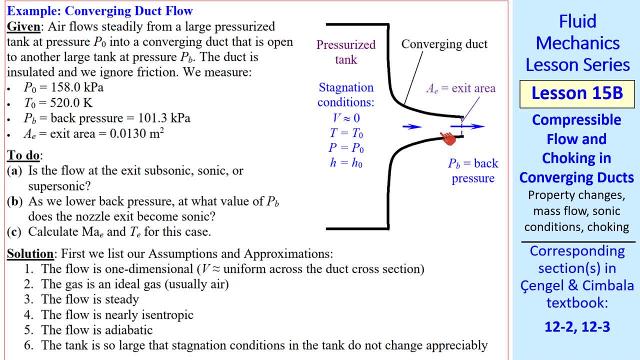 Air flows from this large pressurized tank through a converging nozzle We give P knot, T knot and the back pressure And also the exit area. We want to know if the flow at the exit is subsonic, sonic or supersonic. 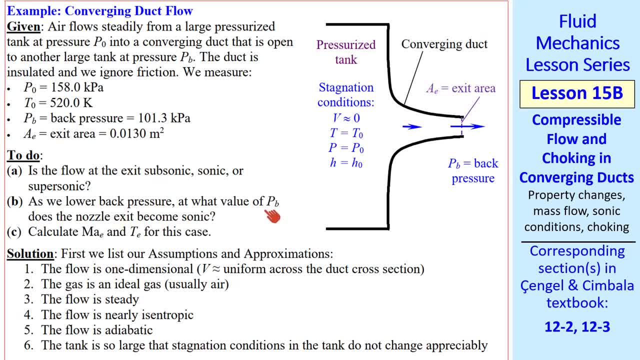 If we keep lowering the back pressure, at what value of Pb will the nozzle exit become sonic? And we want to calculate Mach number and temperature at the exit plane. And for part C, I mean at the given conditions, not when the flow becomes sonic. 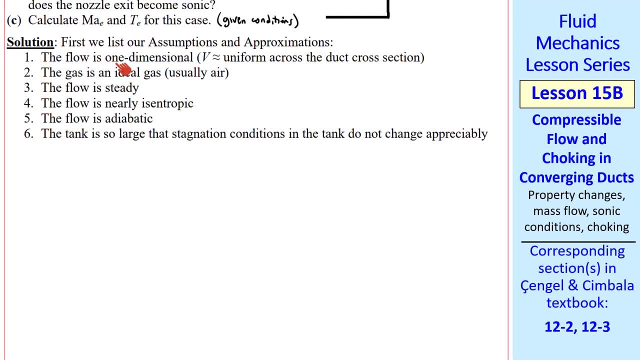 Well, let's list our assumptions and approximations: 1D flow, ideal gas, steady, nearly isentropic, adiabatic. We also assume that the tank is so large that these conditions do not change as flow is escaping. 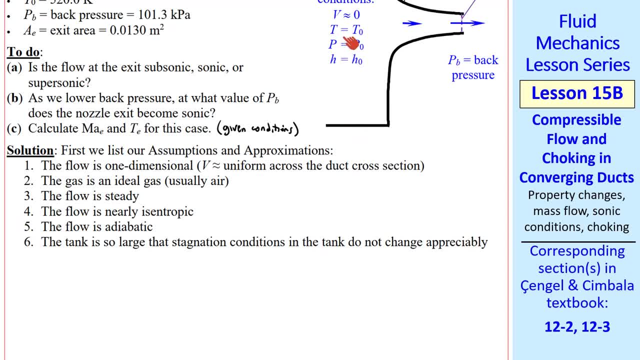 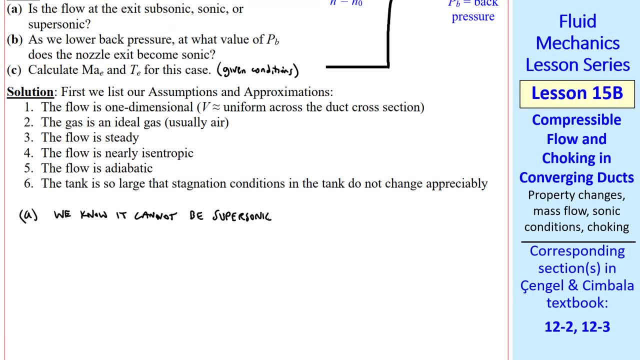 Or imagine that we have a compressor that keeps compressing the air so that T knot and P knot remain the same. Part A: we know that the flow cannot be supersonic, as we discussed above, So that one is definitely not the case. But is it subsonic or sonic? 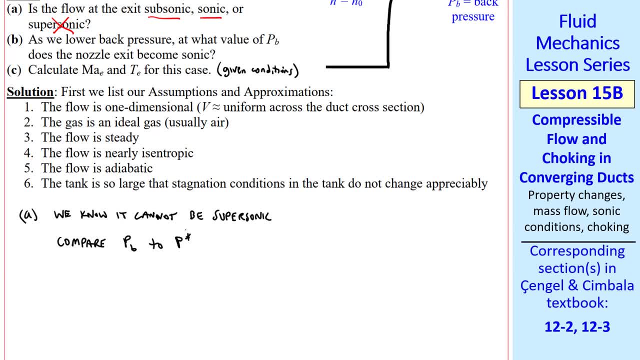 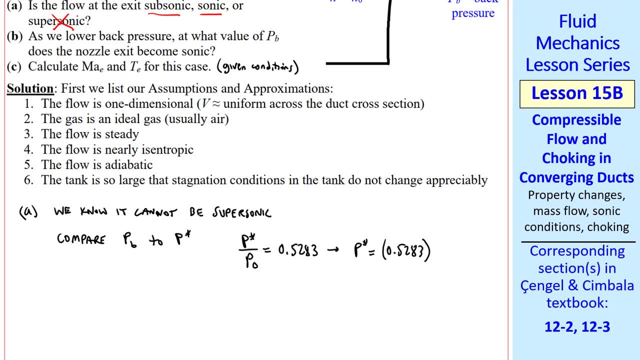 To find out, we compare Pb to P star. For air, P star over P knot is 0.5283.. So P star is 0.5283 times our given value of P knot. So P star is 83.47 kPa. 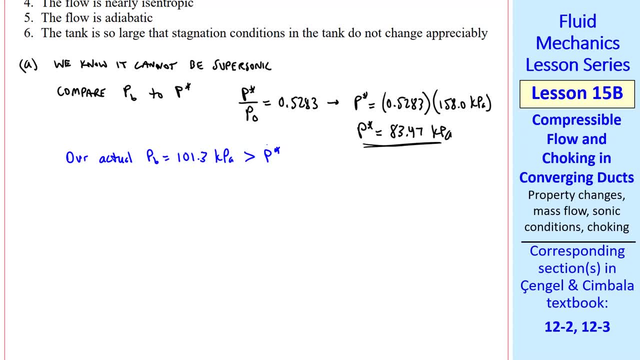 But our back pressure is larger than this. So we have the case of Pb being greater than P star. So this flow is subsonic everywhere and not choked. For Part B, as we discussed if Pb were less than or equal to P star, 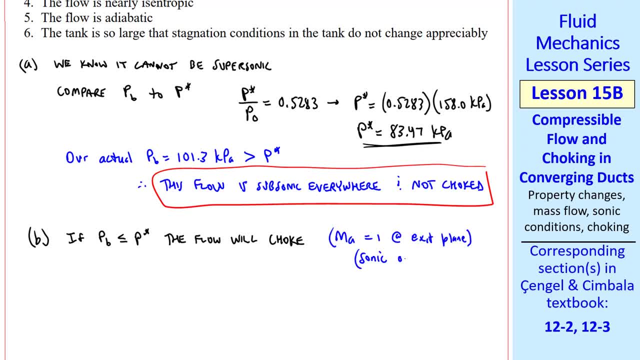 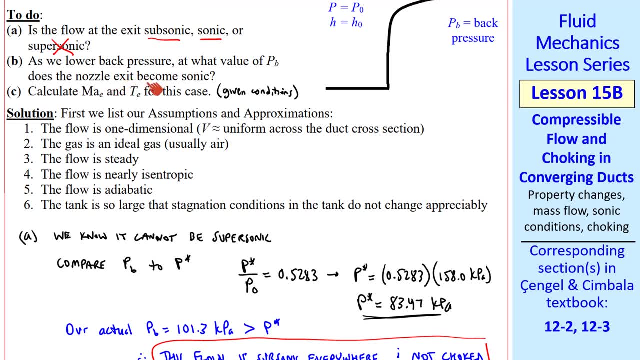 the flow would choke. So the conditions will be sonic or critical at the exit plane. So the answer to Part B: at what value of Pb does the nozzle exit become sonic? at Pb equal P star, which is 83.47 kPa. 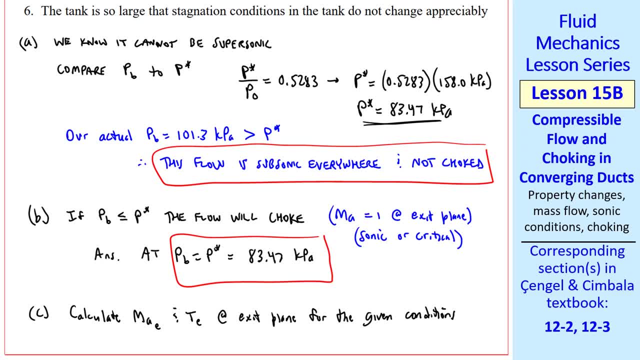 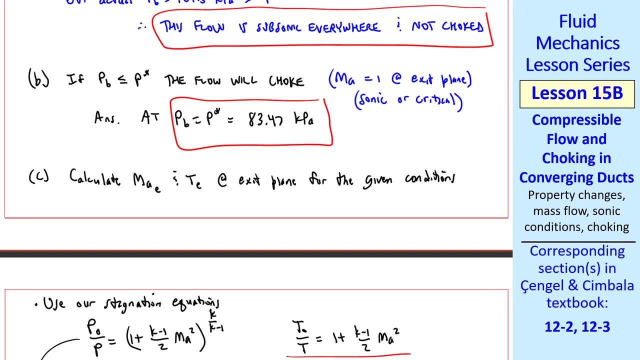 For Part C, we are to calculate Mach number and temperature at the exit plane for the given conditions. I start by using our stagnation equations for P knot over P and T knot over T. We apply these at the exit plane where P equal Pb equal Pe. 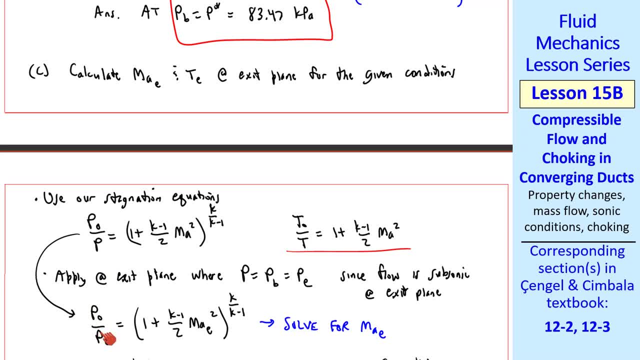 since the flow is subsonic at the exit plane. So I let P equal Pe and Ma equal Mae at the exit plane. I can solve this equation now for Mae, the Mach number at the exit plane. This involves a little bit of algebra. 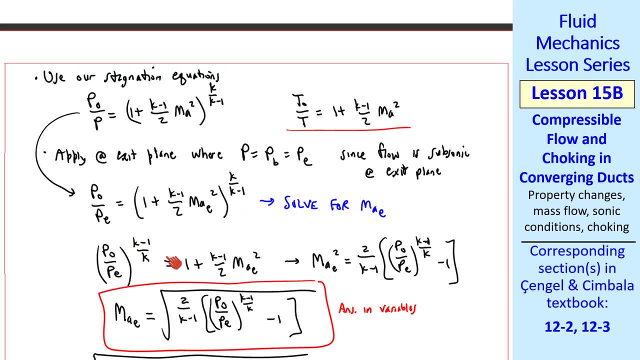 I take both sides to the k minus 1 over k power to get rid of this exponent on the right hand side. Then I solve for Mae squared and take the square root to get Mae. This is my answer in variables. We plug in the numbers. 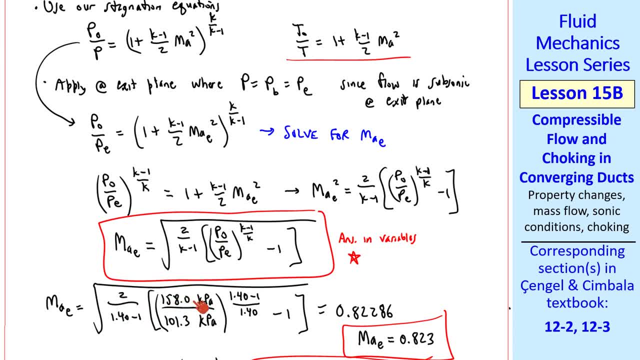 2 over k minus 1, P knot was given and Pe equal Pb, which was also given, and then k minus 1 over k minus 1, square root, I get 0.82286 and I report my final answer to three digits: 0.823.. 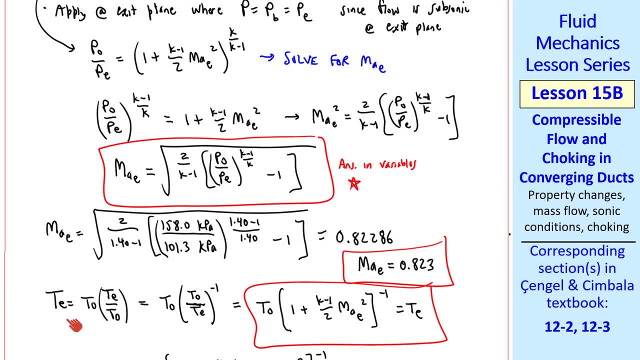 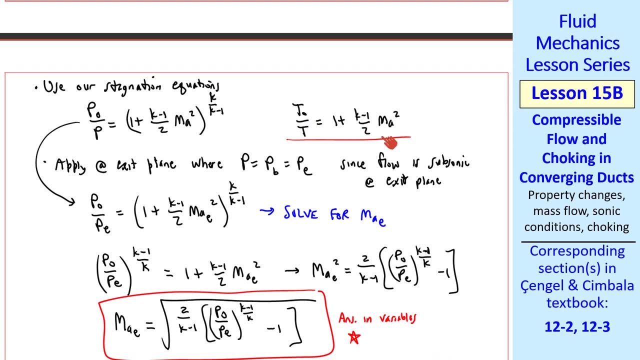 To calculate temperature at the exit plane Te. I write: Te equal T knot times Te over T knot, or T knot times T knot over Te, to the minus 1, since we have an equation for T knot over T. So let T equal Te and Ma equal Mae. 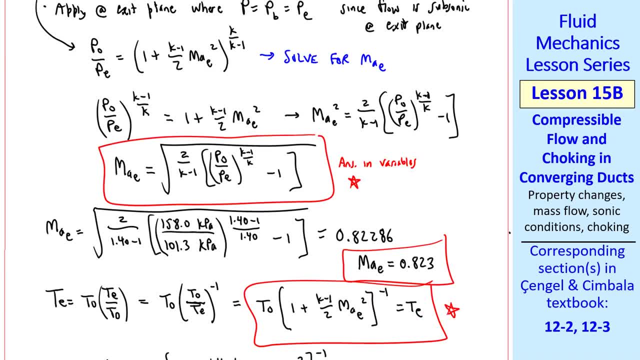 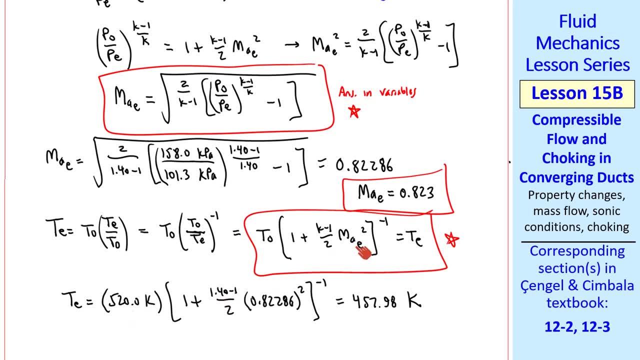 and I get this equation, which is our answer, in variables for Te, Plugging in the numbers: T knot was given 1 plus k minus 1 over 2 times Mae squared, and I'll use all five digits I have there, Then the whole thing to the minus 1. 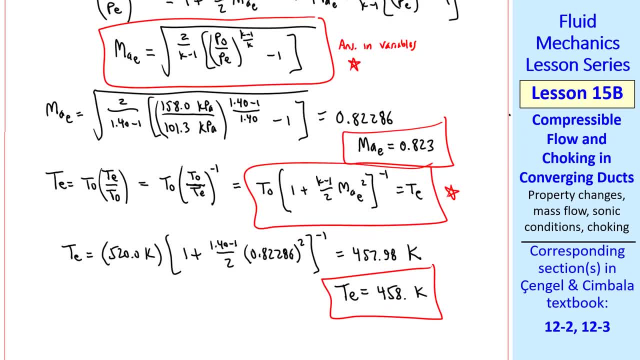 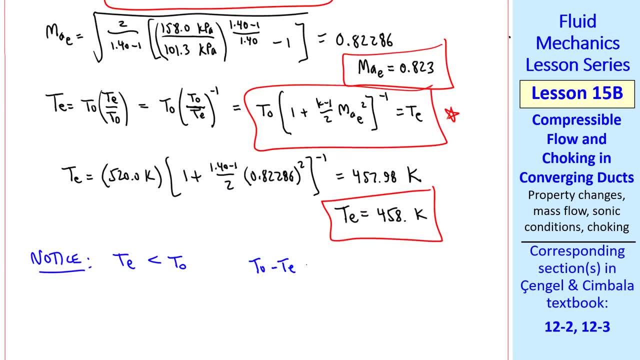 and I get 457.98k. My final answer to three digits is Te equal 458k. Notice that Te is less than T knot. The temperature has dropped by 62k or 62 degrees C. That's a significant drop in temperature. 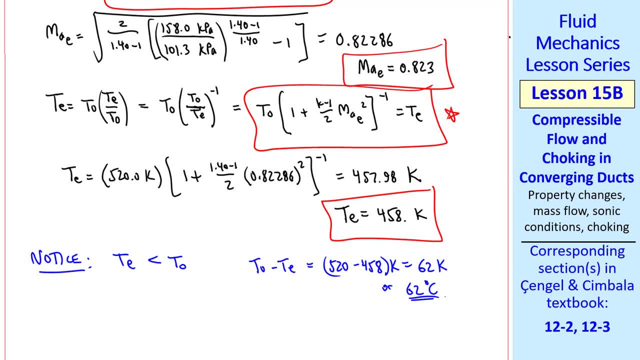 That's why, for example, if you push the little valve in on your bicycle tire and let the air out, the air will feel very cold to your finger, since we can approximate the tire as our pressurized tank and that little protrusion with the valve- 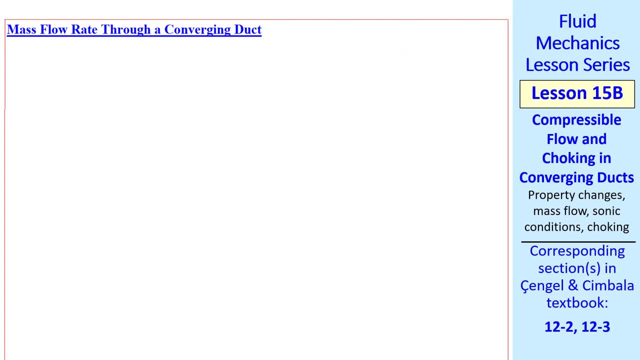 as a converging duct. Now let's consider the mass flow rate through a converging duct Again. assuming that this flow comes from a large tank that is pressurized, While M dot is rho VA anywhere in the nozzle, we can apply that at any x location. 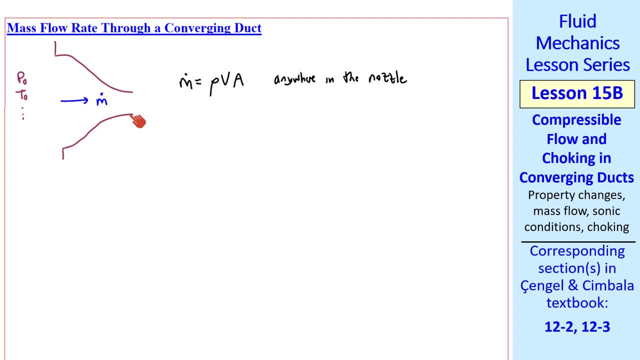 We typically take the exit plane, since we usually know the conditions there. Well, let's work on this equation from the ideal gas law: P equal rho RT, So rho equal P over RT. So we write that, in place of rho, Mach number is V over C. 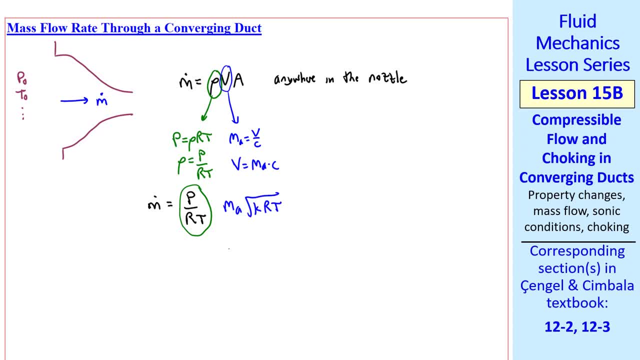 So V, equal MA times C, And C is the square root of krT, So we replace V by this expression And A just comes along for the ride. We can combine the R and the T terms under one square root, So M? dot is PAMA. 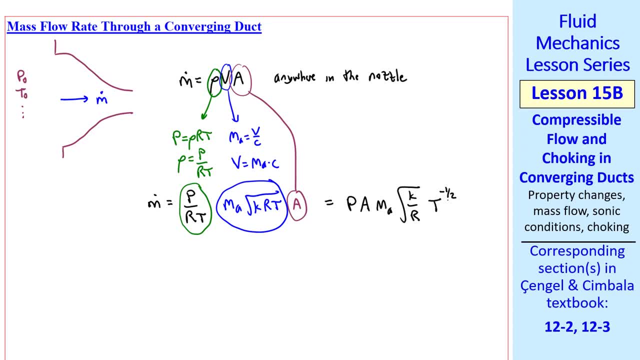 square root of K over R times temperature to the minus one half. We can massage this equation by using our ratios: Instead of P, we use P over P naught times P naught, And instead of T we use T over T naught times T naught. 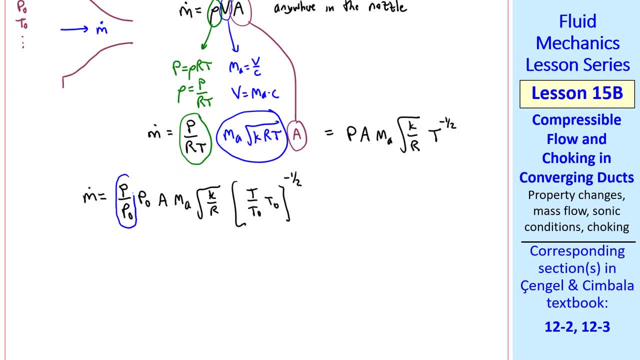 And that raised to the minus one half power. Now we can use our stagnation equations for these two ratios. This is our equation for P over P naught And this is our equation for T over T naught, And we finish off the equation. 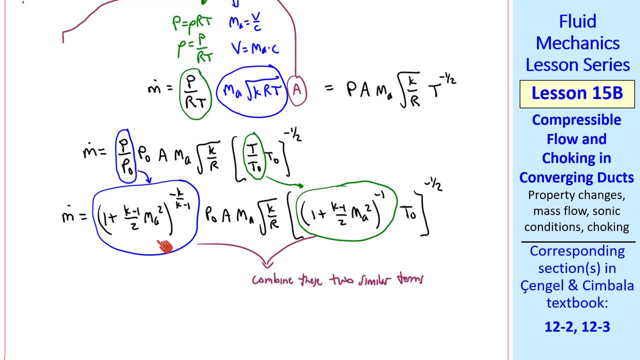 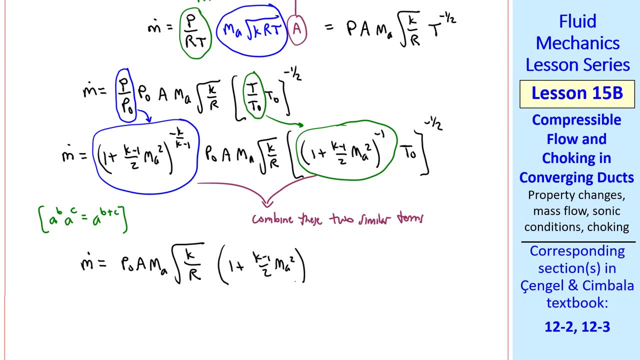 We can combine these two similar terms, since the part in parentheses here and here is the same. We just have different exponents. You should remember this identity from math class. So finally, we have rearranging M dot equal P naught AMA, square root of K over R. 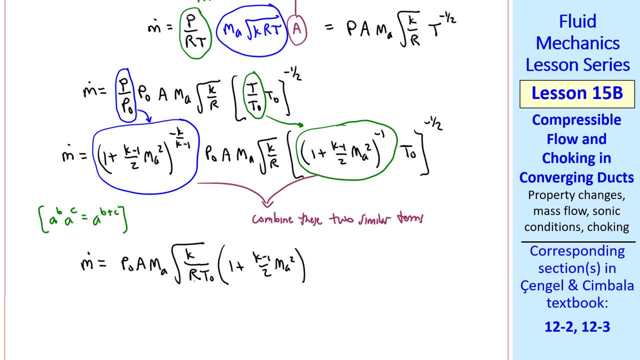 one plus K minus one over two. MA squared, And I put the T naught under the square root sign, And the combination of these two exponents, after a little bit of algebra, is negative: K plus one over two, K minus one If the flow is choked. 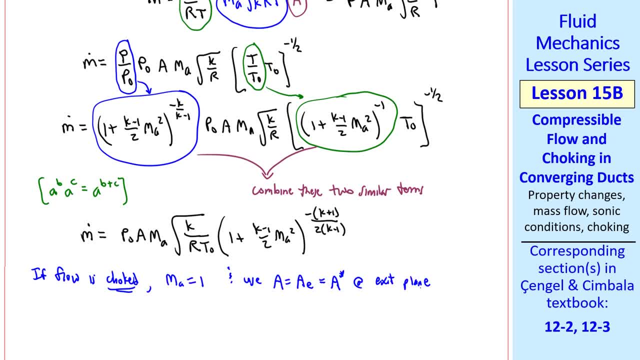 MA equal one and we use A equal AE equal A star at the exit plane, where we define A star as the critical area where the Mach number is one, since the flow is choked. Note that this equation is a general equation, whether the flow is choked or not. 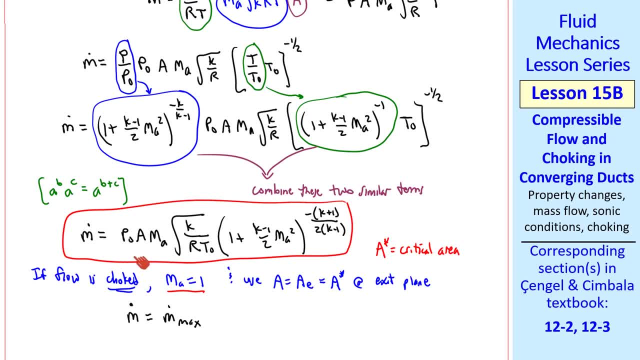 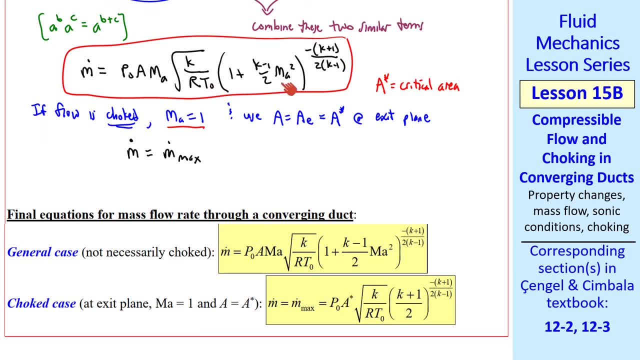 When the flow is choked, the M dot is M dot max and we can simplify this equation. I type these equations up. Here is the general case, which is the equation I derived here. And when we set MA equal one and A equal A star, 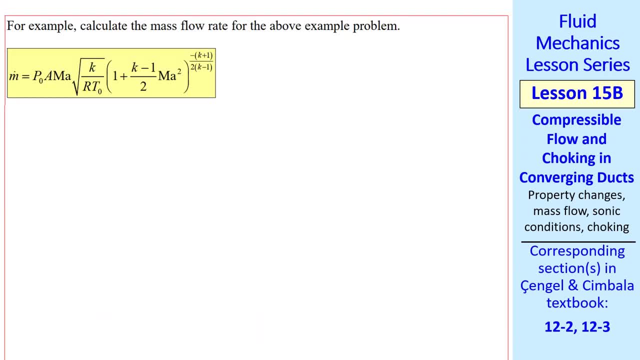 it simplifies to this equation. Finally, let's do an example, namely calculate the mass flow rate for the above example problem. I repeat the equation here. so we plug in the given values and let K equal 1.40 for air, M dot equal P naught. 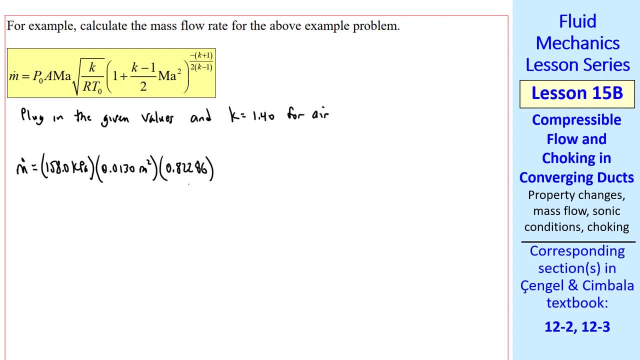 The Mach number at the exit plane. I should mention that we are using the general equation. since this flow is not choked, K over R and T naught and we must be very careful with our units, I'll put in two unity conversion ratios under the square root sign. 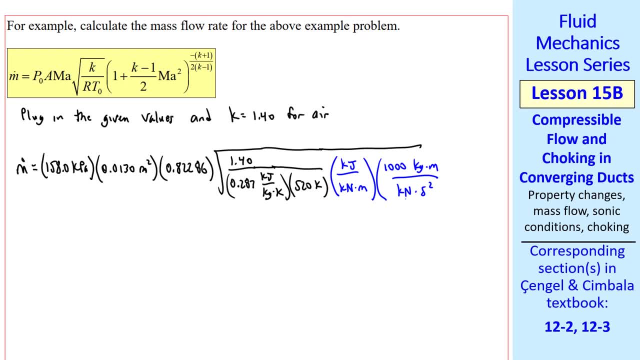 A kilojoule is a kilonewton meter and a thousand kilogram meters is a kilonewton. second squared Now we have this part of the equation left: One plus K minus one over two, Our Mach number at the exit plane. 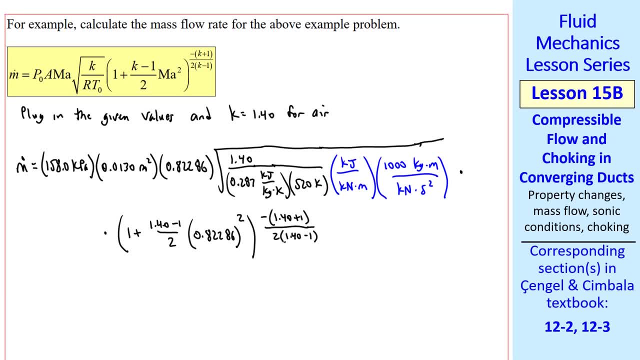 squared and the exponent where K is 1.40.. I need one more unity conversion factor and we check our units. KPA cancels Meters. cancel Kilojoules. cancel K cancels These two kilonewtons, cancel this one. 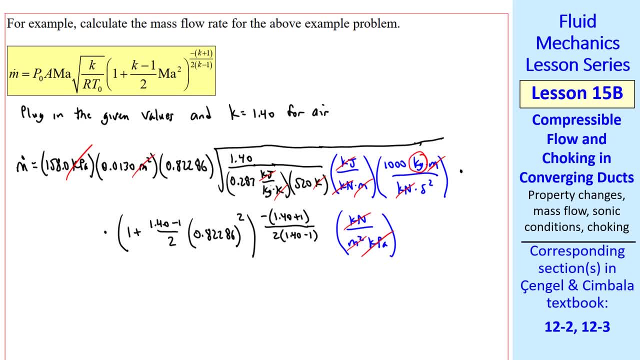 This meter squared cancels this one And we are left with a kilogram and another kilogram square root, which is kilogram, over second squared square root, which is second. So we get 3.65 kilograms per second. This is an exercise in unity conversion factors. 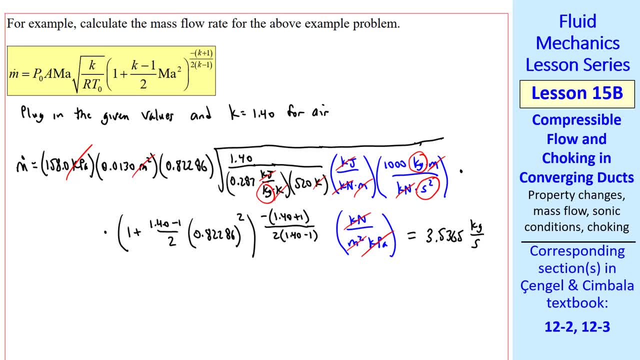 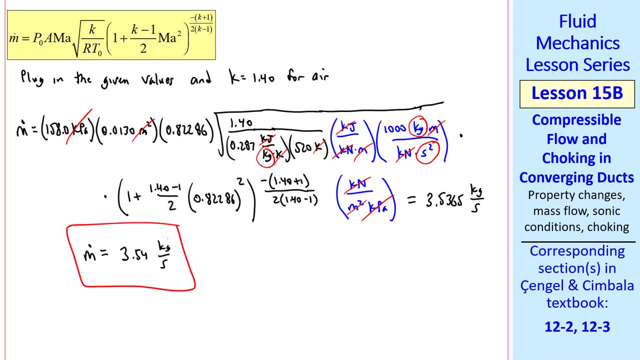 but if you do everything correctly, the units all work out and we get kilograms per second as our final answer. Finally, to three digits, we get m dot equal 3.54 kilogram per second. I'll leave it as an exercise to calculate m dot max. 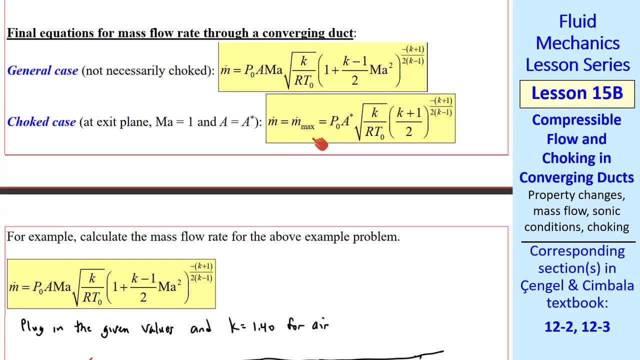 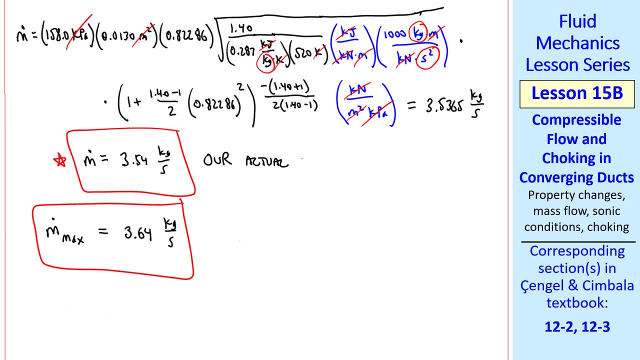 You should get 3.64 kilograms per second. That would be using this equation and being similarly careful with your units. so this mass flow rate is our actual flow rate and this m dot max would occur if Pb were less than P star. In other words,